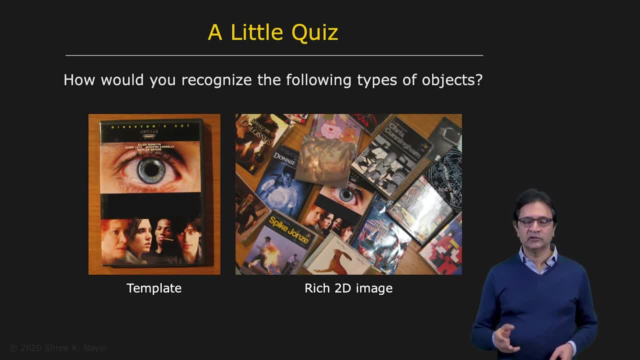 first instinct may be to use something like template matching. We know how to do that. We know how to do that using normalized correlation. But the problem is that the object doesn't show up exactly in its original form in the image. It's actually rotated in the image. 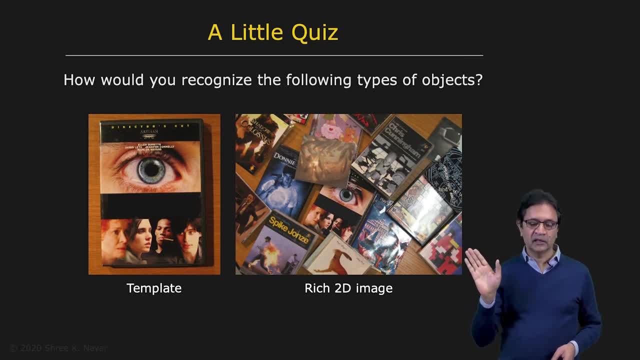 and is also magnified differently. In other words, it has a different scale in the image, And so, in order to deal with rotation and scale, you might have to then create lots of templates of this object under different rotations and scales and apply each of one. 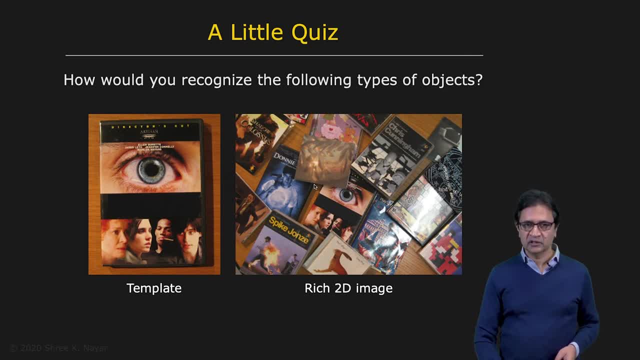 of those to the image, And so in order to do that, you might have to create lots of templates of this object under different rotations and scales and apply each of one of those to the image, which would be computationally just impractical. But actually the harder problem here is occlusion. 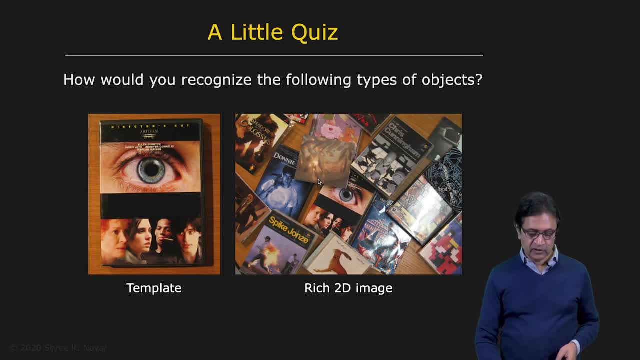 You see that this object is actually obstructed by other objects. This is hard, And so dealing with that using template matching might require you to actually create a lot of little templates here from this object and then apply each one of those and make sure that in your final 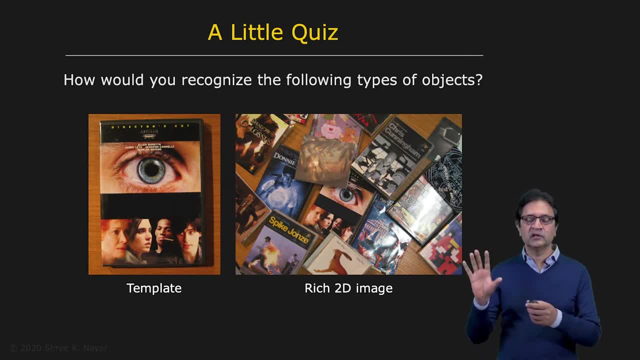 output. there are enough templates of this object that appear in the image, And so you want to get a lot of information about how you're going to apply these templates in this image. So by doing these things, you're going to be able to actually create lots of other templates. 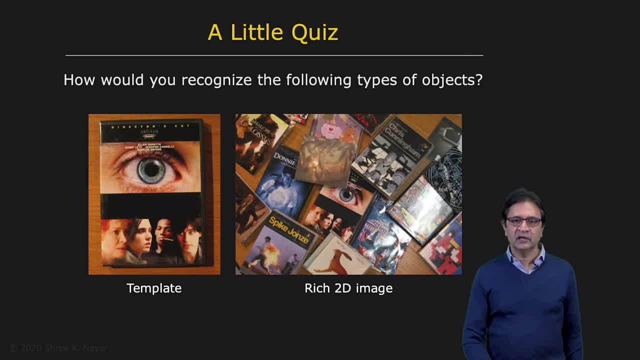 that seem quite much like this object. So the first thing we have to do is to create a template. You can do that by typing the format header and then the format header and the format header is set by default And then, if you want, you can change it. So if you want to use this, you can choose the. 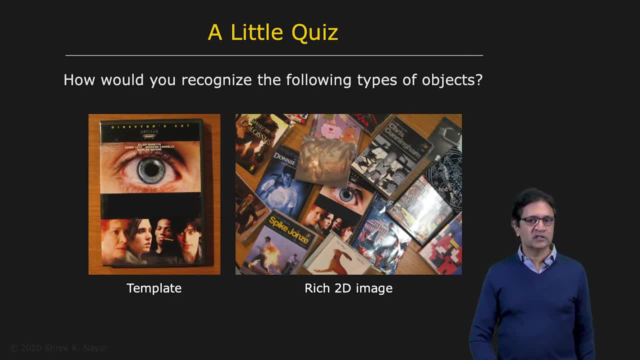 object that you want to use, So you can. actually, you know, if you have your own template, you can use this template here. So you want to create a template and you want to say, okay, we want to be able to use this. 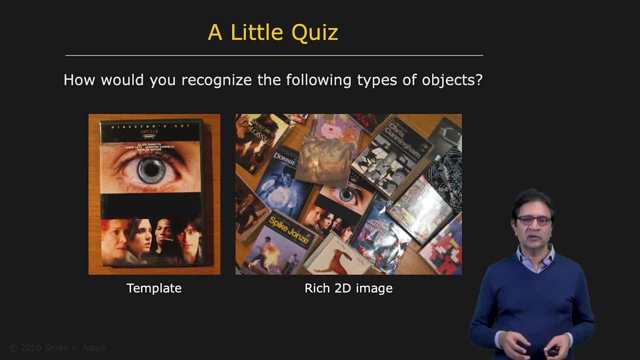 template here, And then you want to do it in a very different way than you could not. You can do something about it, like a simple document do is somehow extract directly from this image that's given to you some very descriptive, unique features. 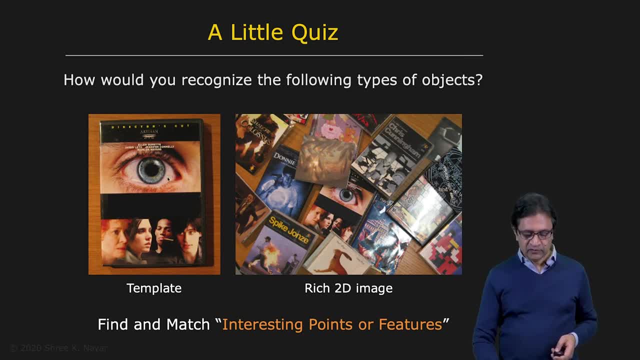 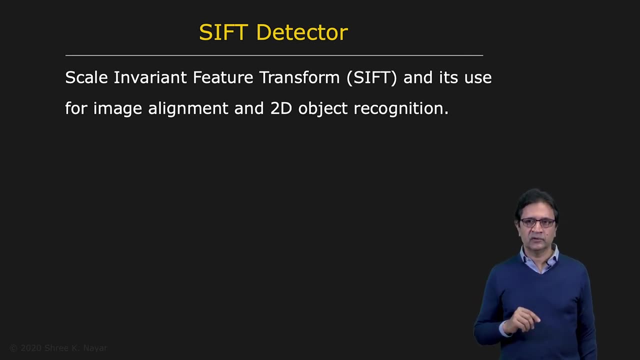 So if we can find these features and if we can find the same features in this image, then we can match them and we can recognize the object. And that's exactly what the SIFT detector does. So SIFT is short for Scale Invariant Feature Transform. 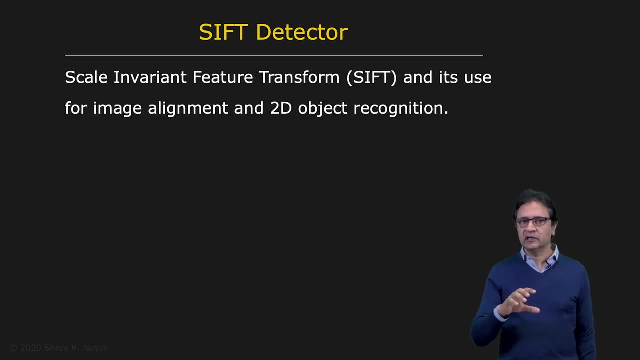 And we'll describe the theory behind the SIFT detector and its implementation and also show how it's used to solve some interesting vision problems. simple vision problems such as image alignment and stitching, as well as 2D object recognition. So we're going to start with asking the question. 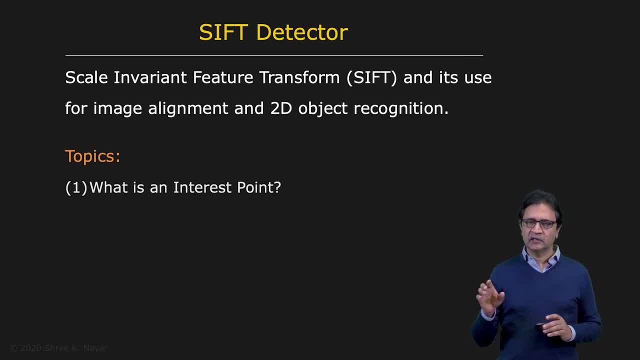 what is an interest point? By the way, this is an area of research in computer vision that has a long history. I think the term interest point is really came from Hans Moravec back in the late 1970s. He was looking at what are interesting points. 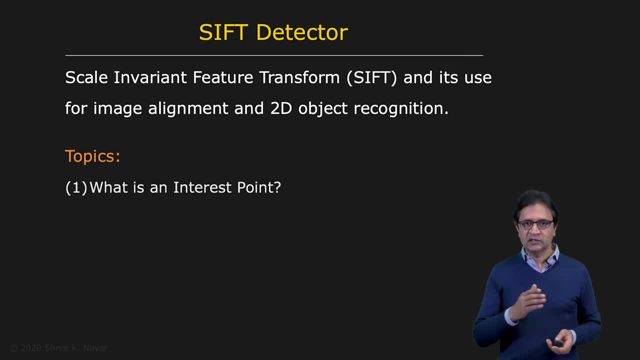 in the context of robot vision, And since then there's been a lot of work in this area. that goes to say that edges and corners are not really interesting enough points for a lot of applications. We need things that are a little bit more descriptive. 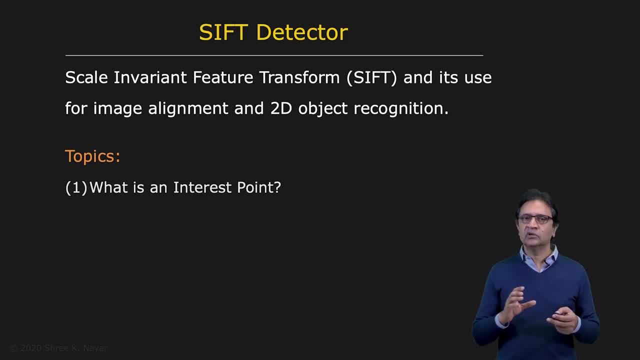 And what has been realized over time is that some notion of a blob which has some local appearance within it is potentially a very good interest point to try and find and to use for matching as well. So we'll talk about detecting blobs. By the way, I should mention once again: 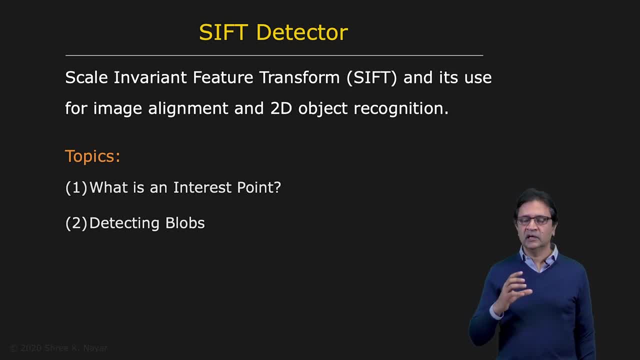 that the term blob is being used very loosely here. It's a patch with a local appearance, And we'll use derivatives of images to actually detect blobs, very much like what we did with edge detection. We'll create a theory for blob. We'll create a theory for blob detection. 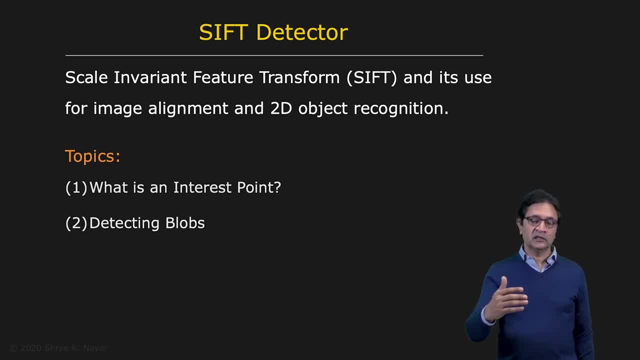 And what's nice about this theory is that it can detect blobs over multiple scales. It can handle not only the position of the blob but also the magnification of the blob, Because an object can appear at many different magnifications depending on its depth from the camera. 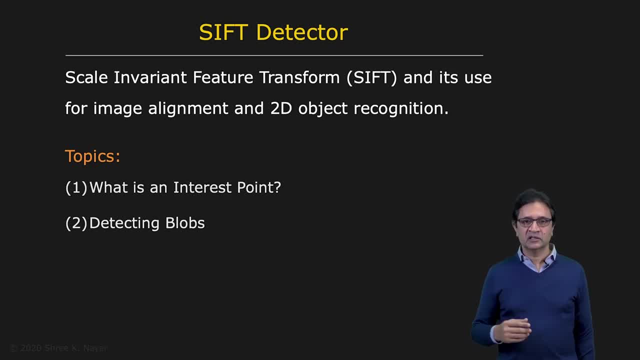 So you have to be able to deal with scale, And so this blob detection theory handles scale in a very simple way, And using this theory, we are going to develop the SIFT detector, which was proposed by David Lowe. It's a very clever, very clean implementation. 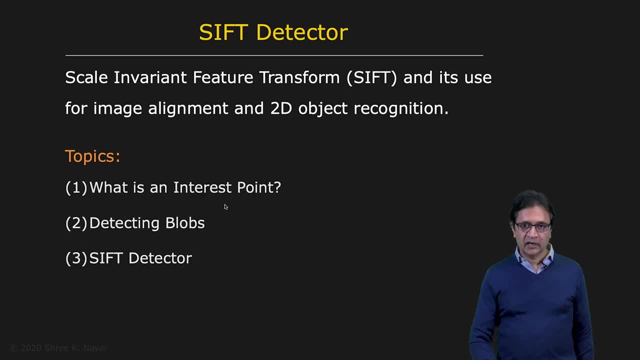 of blob detection And we'll see how it's done, And we'll also show that it is very robust and reliable in terms of extracting interest points from images. Now that brings us to the point where we can actually extract these points in any image that's given to us. 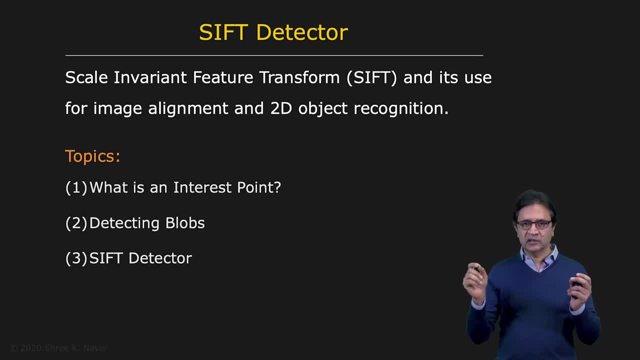 But in order to match a point in one image to a point in another image, in other words an interest point in one image to an interest point in another image, you really need some kind of a signature that describes the local appearance around the point.